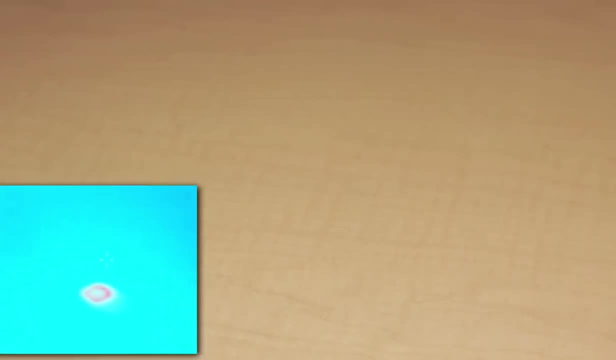 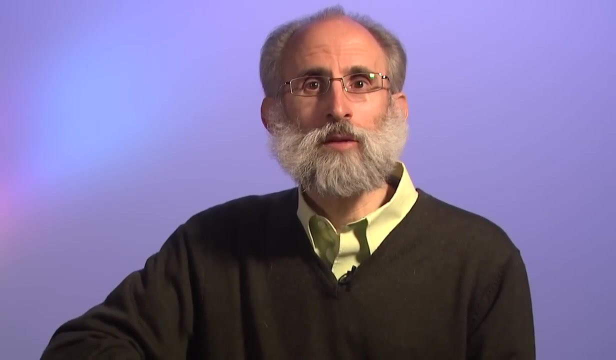 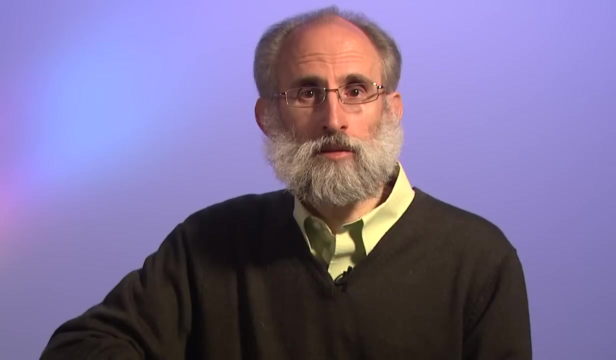 But if we remove the cup of tea, the counter top eventually returns to room temperature. We say that the counter at room temperature is a stable equilibrium. In this video we discuss the world from the perspective of equilibrium and stability and, in particular, linear stability. 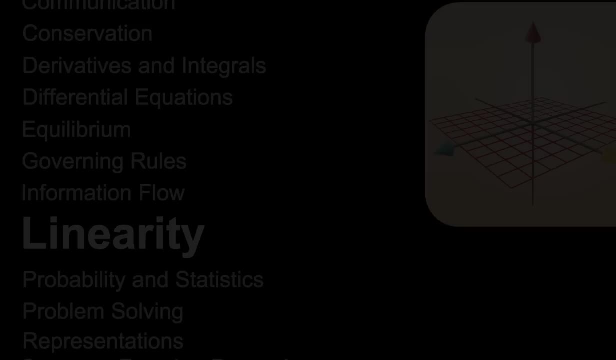 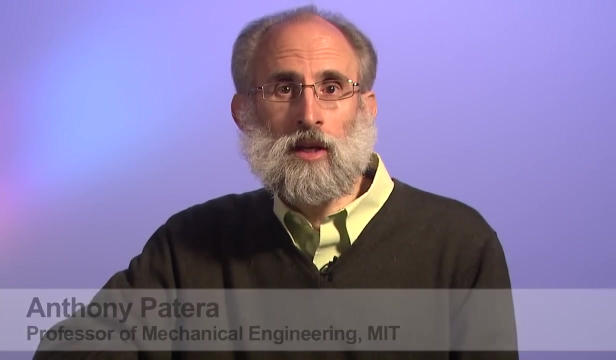 This video is part of the linearity video series. Many complex systems are modeled or approximated as linear because of the attendant mathematical advantages. All the world is an initial value problem and the matter merely state variables. However, and less poetically, there are alternative interpretations of physical. 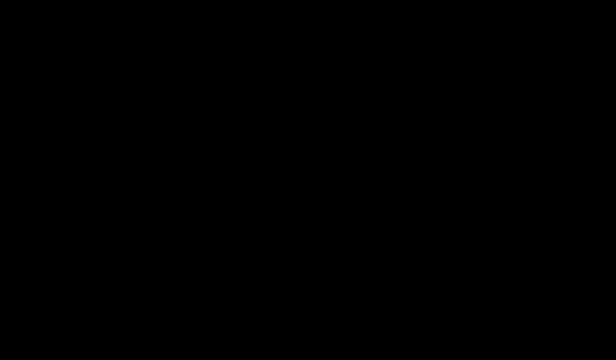 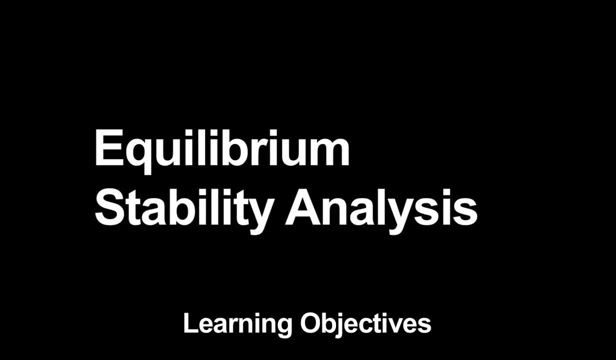 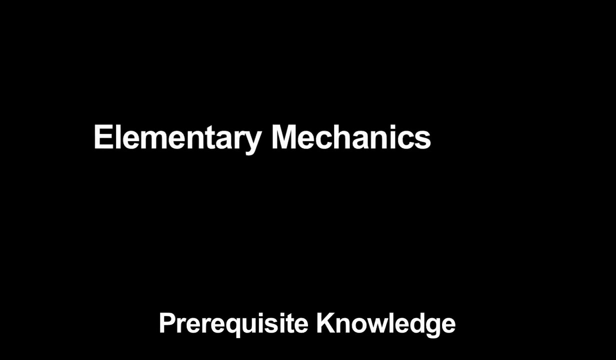 and indeed social systems. that can prove very enlightening. The purpose of this video is to introduce you to the framework of equilibrium and stability analysis. We hope this motivates you to study the topic in greater depth. To appreciate the material, you should be familiar with elementary mechanics. 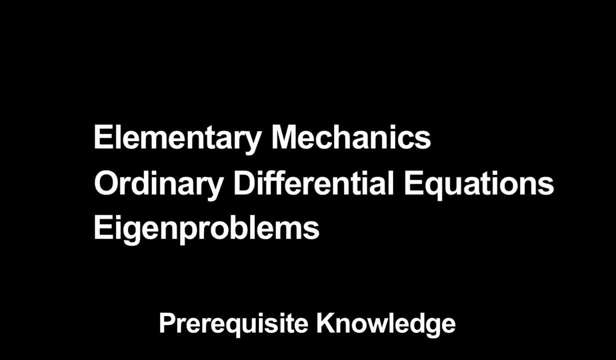 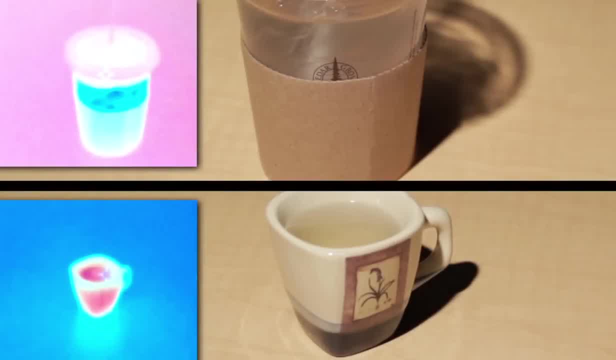 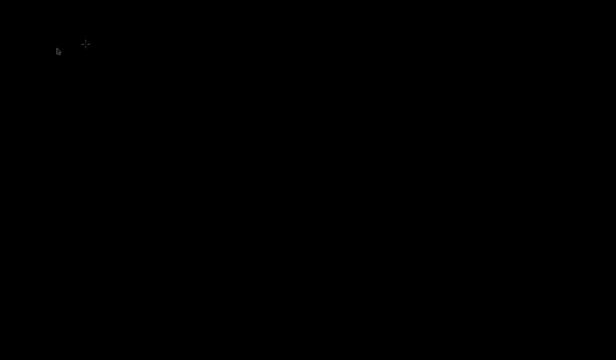 ordinary differential equations and eigenproblems. Let's look at the iced drink and hot teacup example from the perspective of equilibrium and stability. In this example the governing partial differential equation is the heat equation shown here. At equilibrium, the solution of the governing equations is time independent. 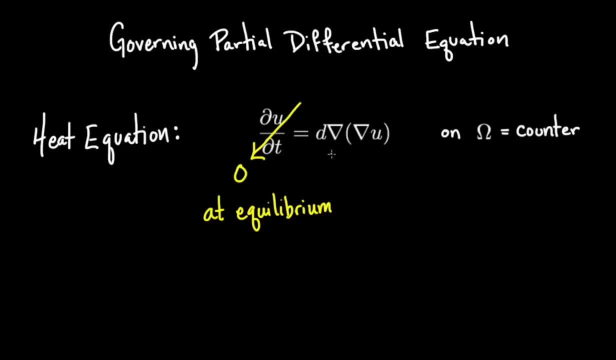 That is, the partial time derivative is zero. This tells us that the del squared temperature term must also be zero and therefore the partial time derivative is zero, Which is only possible, given the boundary conditions, if the entire counter is at room. 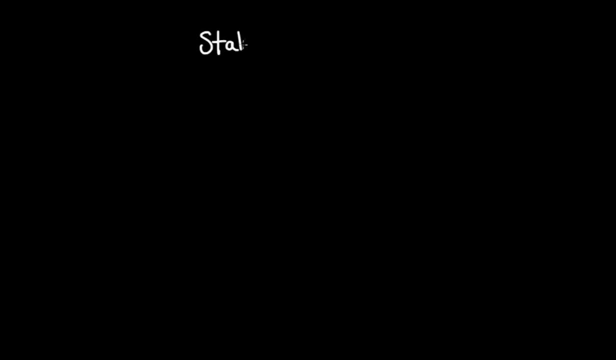 temperature Stability refers to the behavior of the system when perturbed from a particular equilibrium, here the uniform counter temperature. A stable system returns to the equilibrium state. An unstable system departs from the equilibrium state. We say that this equilibrium is stable because if we perturb the temperature by increasing 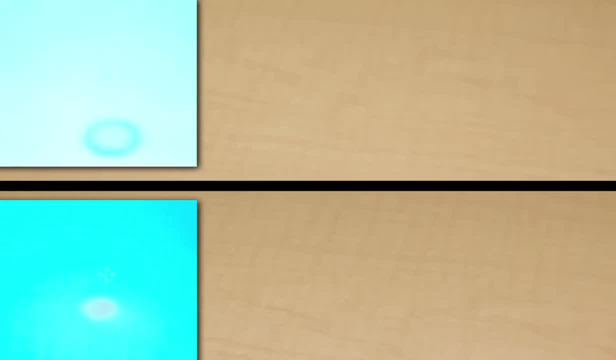 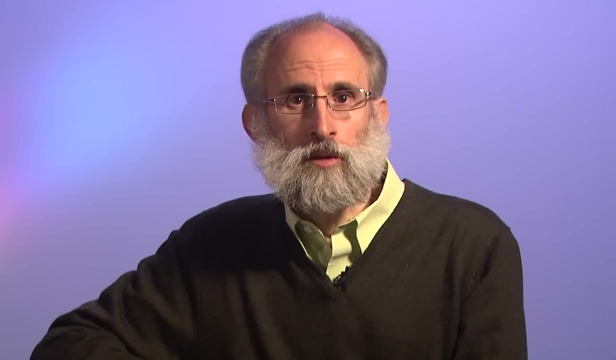 or decreasing the temperature slightly, it will return to room temperature, the equilibrium state, after enough time. Here we intuitively understand from our experiences that the equilibrium is stable, But for other situations we need mathematical methods for determining whether or not equilibria. 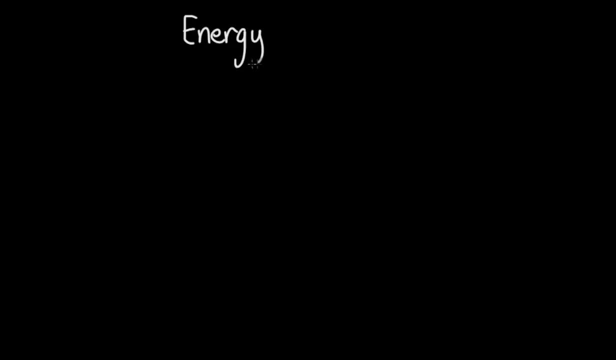 are stable. One way to determine if the equilibrium of this partial differential equation is stable is to apply an energy argument. Manipulation of this heat equation permits us to derive a relationship between the equilibrium and the equilibrium. You can see that the equilibrium is stable. 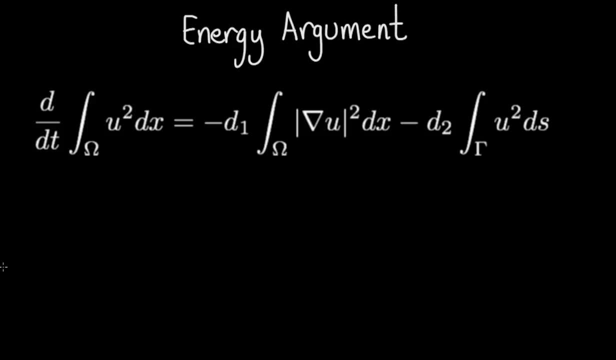 It's stable. The equilibrium is stable. that describes how the mean square departure of the counter temperature from room temperature evolves over time, as shown here. Note u of x is the deviation of the temperature in the counter from room temperature, omega is the counter region and gamma is the counter surface. 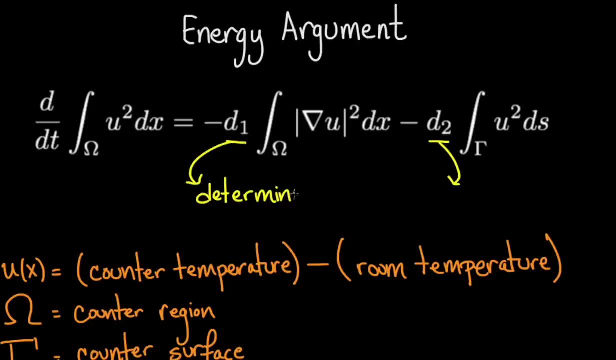 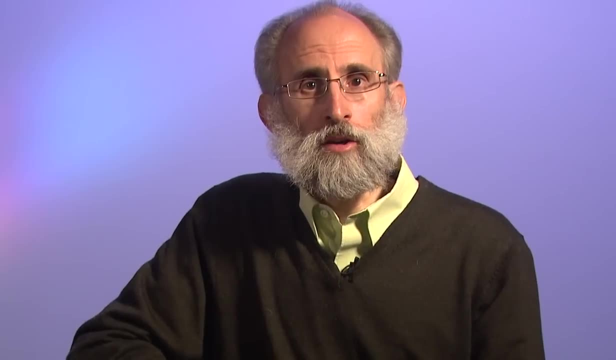 d1 and d2 are positive constants determined by the thermal properties of the counter. Because the right-hand side of this equation is negative, it drives the temperature fluctuations. the integral of ux squared over the counter region to zero. This energy argument is the mathematical prediction of the behavior we observe physically. 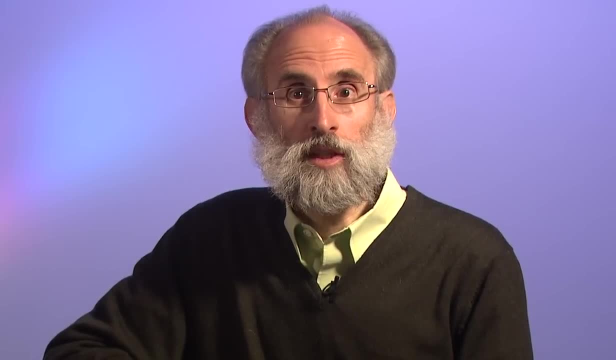 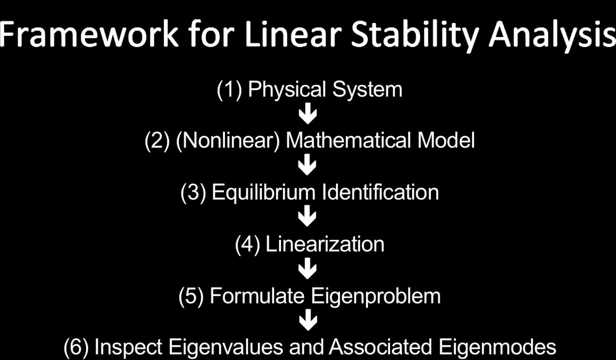 Linear stability theory refers to the case in which we limit our attention to initially small perturbations. This allows us to model the evolution with a linear equation. Linearizing the governing equations has many mathematical advantages. Let's consider the following framework for linear stability analysis. 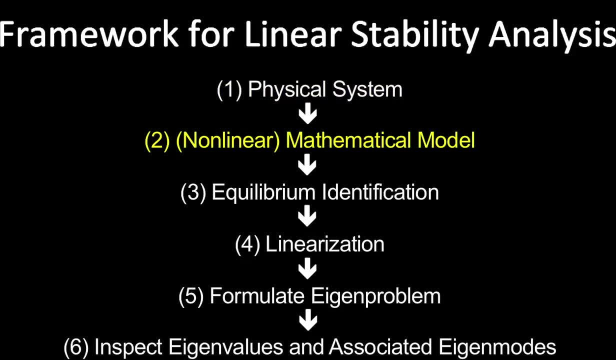 1. Choose a physical system of interest. 2. Develop a typically nonlinear mathematical model. 3. Identify equilibrium. 4. Linearize the governing equations about these equilibria. 5. Convert the initial value problem to an eigenproblem. 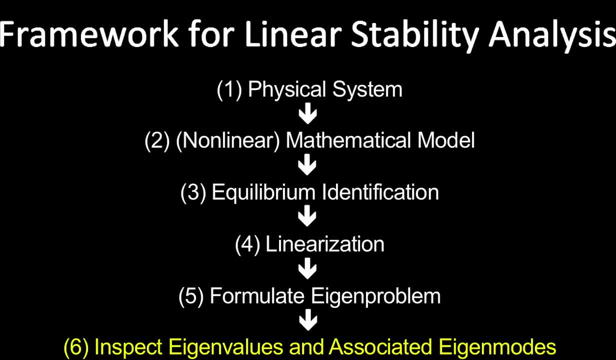 6. Inspect the equation. 7. Identify the equilibrium. 8. Identify the equilibrium. 9. Identify the equilibrium. 10. Identify the equilibrium. 11. Identify the equilibrium. 12. Identify the equilibrium. 13. Identify the equilibrium. 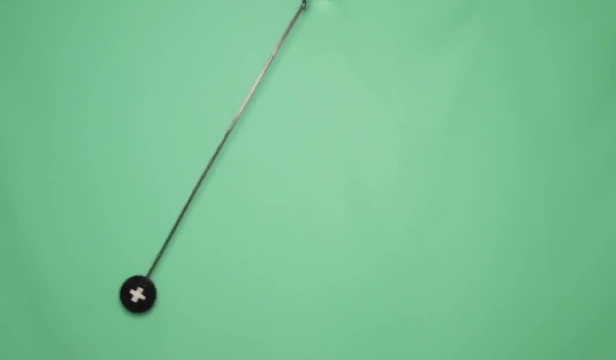 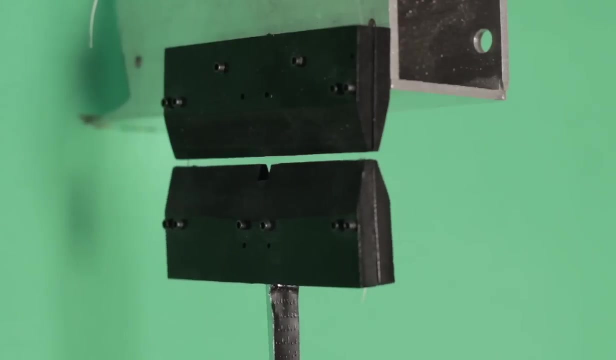 Let's see how to use this framework as we proceed through the example of the real physical pendulum seen here. You see a large bob, the rod and a flexural hinge which is designed to reduce friction losses. Let's now develop the mathematical model. 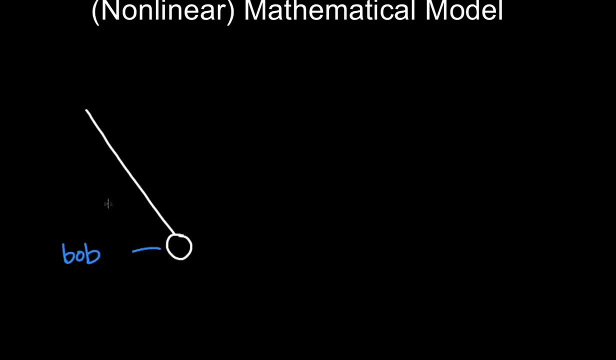 We show here the simple pendulum consisting of a bob connected to a massless rod. We denote the angular position of the bob by theta of its height, by theta of t, and the angular velocity of the bob by omega of t. g is the acceleration due to. 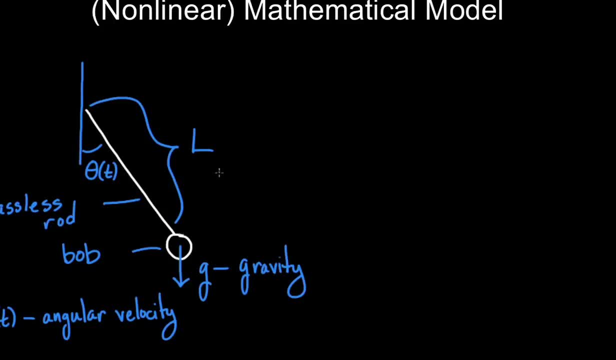 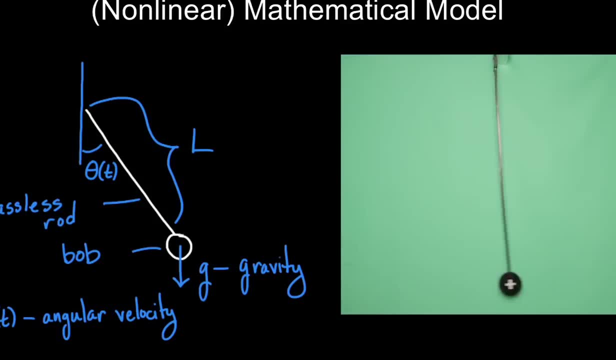 gravity, and L is the effective rod length for our simple pendulum. The effective length L is chosen such that the simple pendulum replicates the dynamics of the real physical pendulum. L is calculated from the center of mass, the moment of inertia and the mass of the compound pendulum. 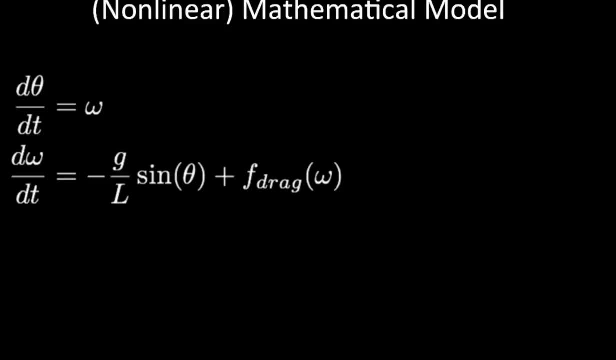 The dynamics may be expressed as a coupled system of ordinary differential equations that describe how the angular displacement and angular velocity evolve over time. These equations are nonlinear due to the presence of sine theta and the drag function. f. drag of omega. The drag function is: 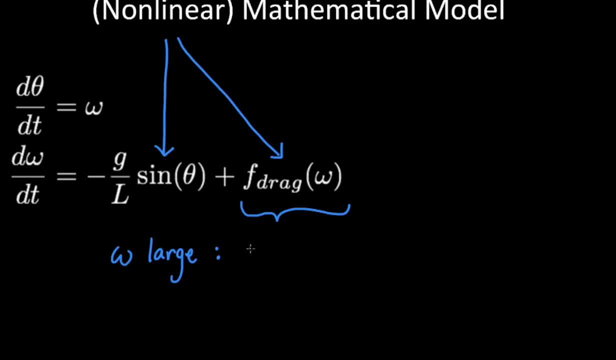 quite complicated. For large omega it is equal to c, absolute value of omega omega, where c is a negative constant. But for very small angular velocities near points on the trajectory where the pendulum is not moving, or at least not moving fast, the drag is given by b. 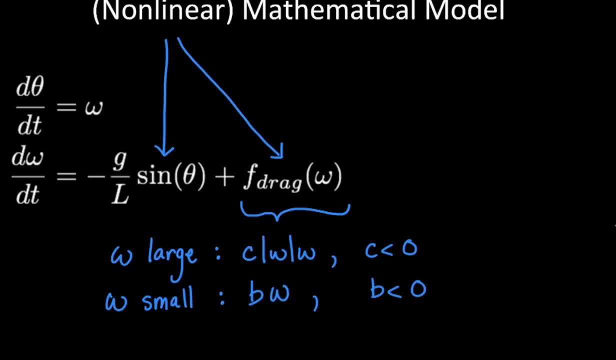 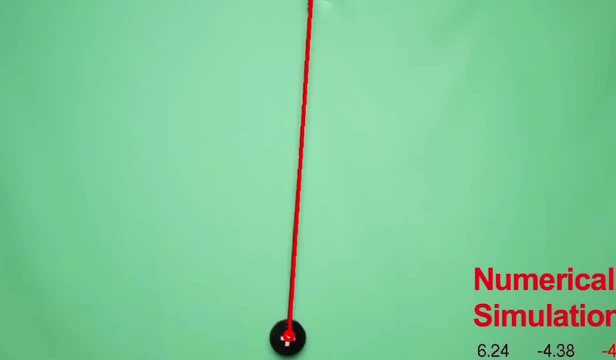 omega, where b is a negative constant. Next, let's explore the validity of this model. Here you see a comparison between a numerical simulation and an experiment, courtesy of Drs Yano and Penn respectively. The numerical simulation is created by calibrating the drag function to the 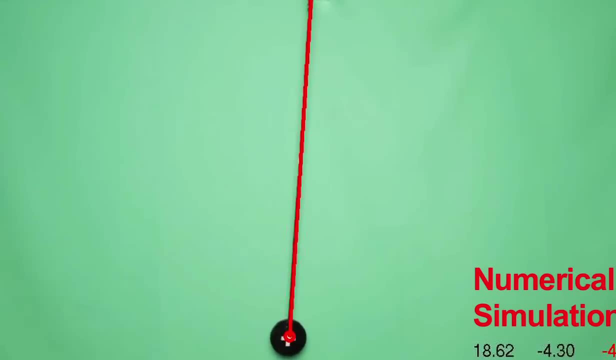 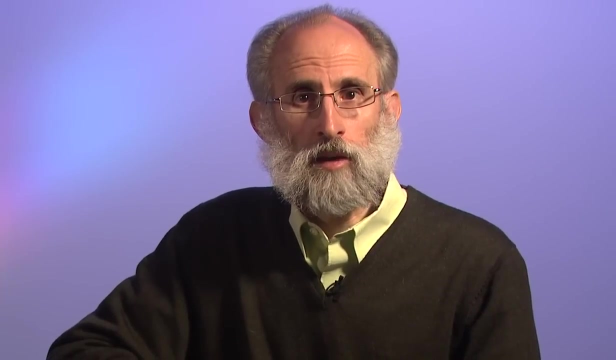 experimental data. The agreement is quite good for both small and large initial displacement. However, because we are fitting the dissipation to the data, this comparison does not truly validate the mathematical model. To validate the mathematical model, we must focus on a system. 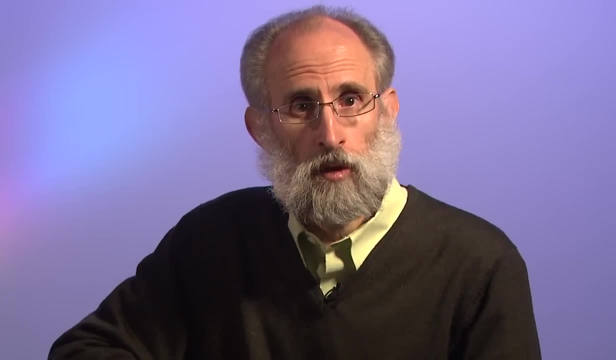 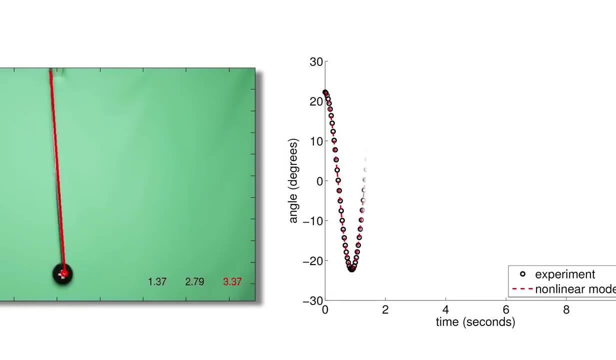 property that is largely independent of the here small dissipation, such as the natural frequency or period of the pendulum motion. A comparison of the natural frequency of the physical pendulum to that predicted by the numerical model shows that the natural frequency of the physical pendulum 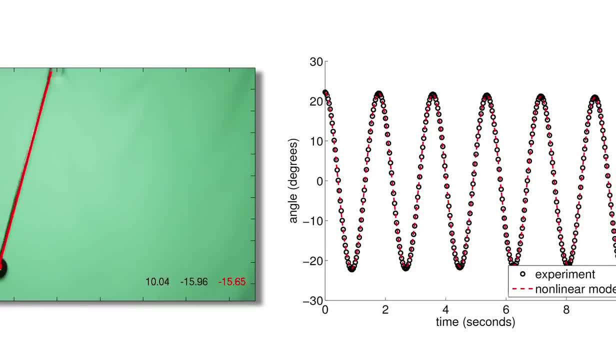 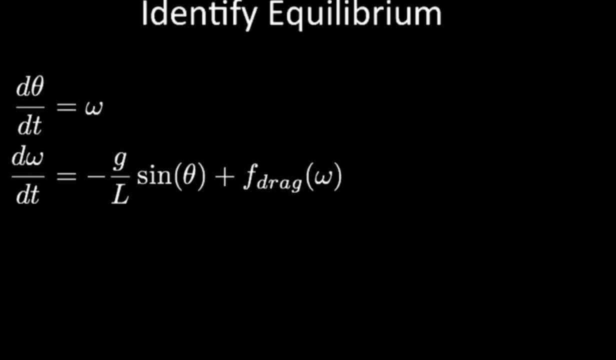 shows that the natural frequencies agree quite well for any initial displacement angle, even large. We now look for equilibrium states, that is, solutions that are independent of time. To find these equilibria, we set the left-hand side of the equations to zero and solve for theta and 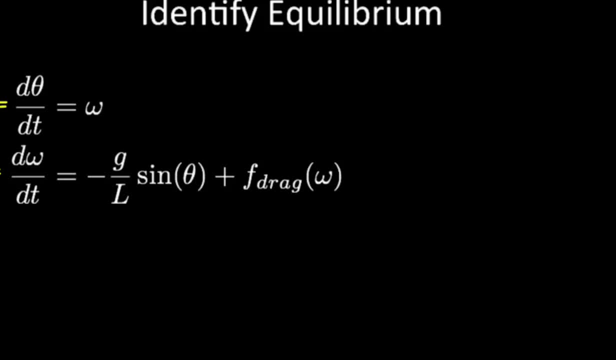 omega, We can readily conclude that there are two equilibria: theta omega equals zero- zero, which we denote the bottom equilibrium, and theta omega equals pi- zero, which we denote the top equilibrium. The mathematical model actually has infinitely many equilibria corresponding. 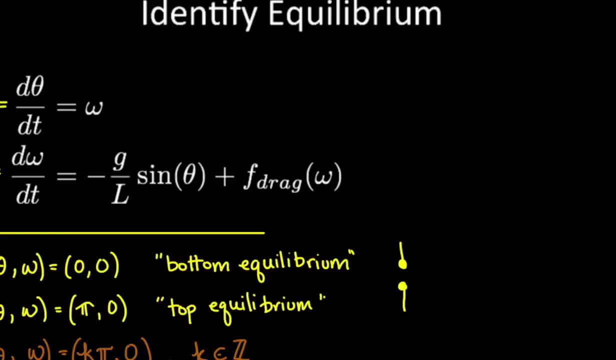 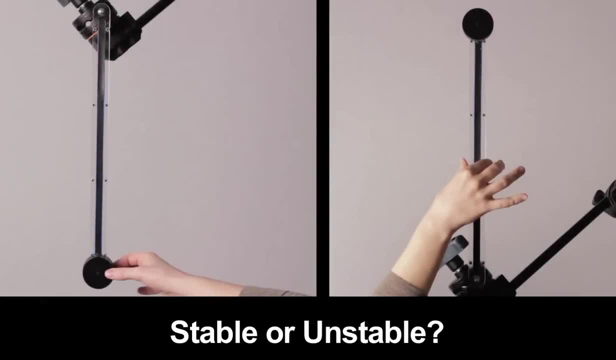 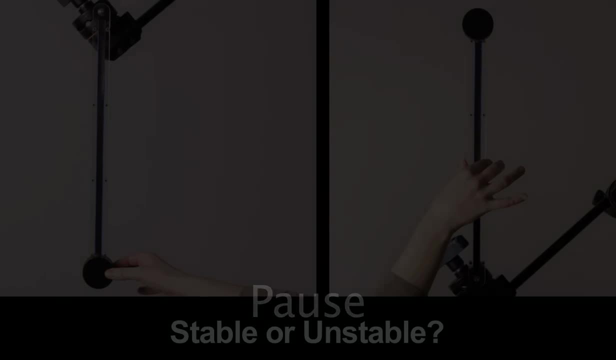 to this, but for our stability analysis two equilibria suffice. Are these equilibrium solutions stable or unstable? You might pause the video and discuss. They are stable if a small nudge will result in a commensurately small bob motion. They are. 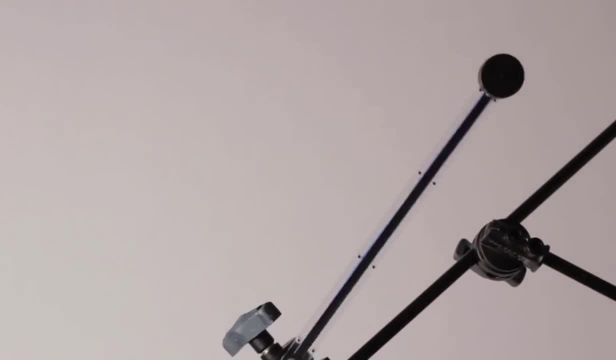 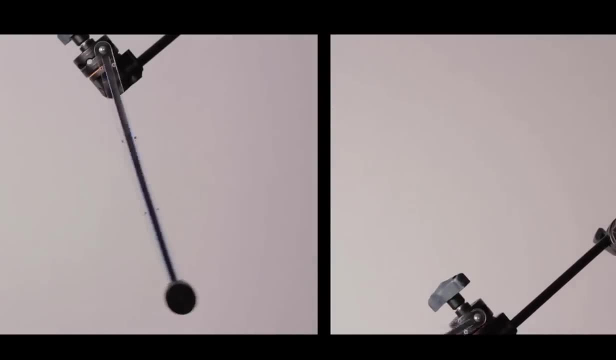 stable if a small nudge will result in incommensurately large bob motion. So we can predict that the bottom equilibrium is stable, the top equilibrium unstable. If our mathematical model is good, it should predict the same behavior as the physical system. 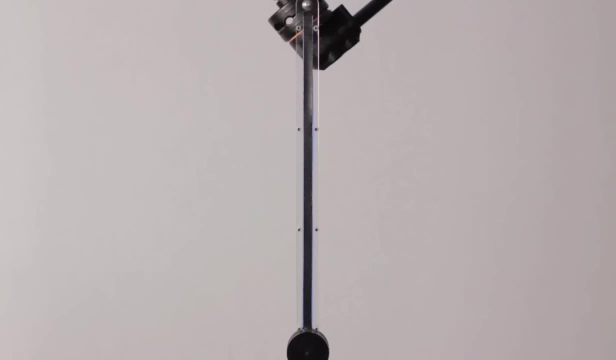 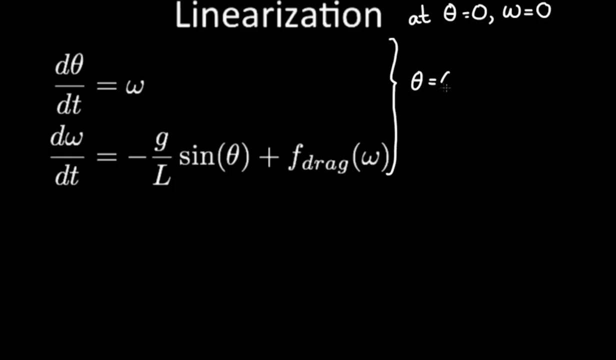 But how do we mathematically analyze stability of our model? Let's work through the linear stability analysis framework. for the bottom equilibrium, theta equals 0 and omega equals 0.. First we linearize the equations about the equilibrium. The linearized equations are only valid near the equilibrium. theta equals 0 and. 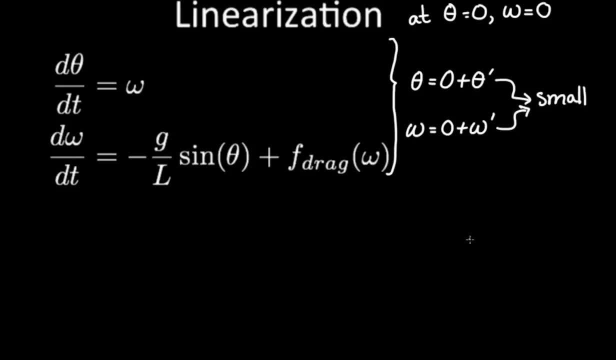 omega equals 0, ie for small displacements, theta prime, with small angular velocities, omega prime. The first equation of our system is already linear, So we only need to worry about linearizing the sine of 0 plus theta prime term and. 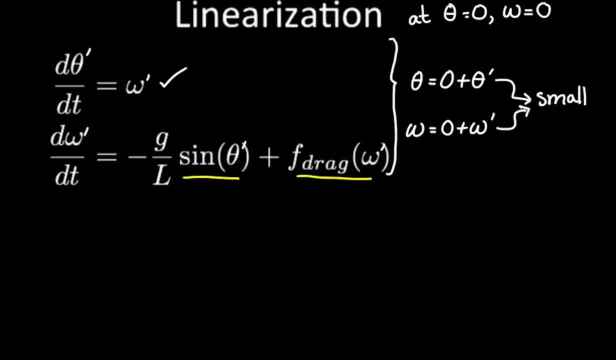 the dissipation term of the second equation for small theta prime and omega prime. What is the linear approximation of sine theta prime about? theta equals 0? You might wish to use a Taylor series and we'll pause the video and allow you to write down your answer. 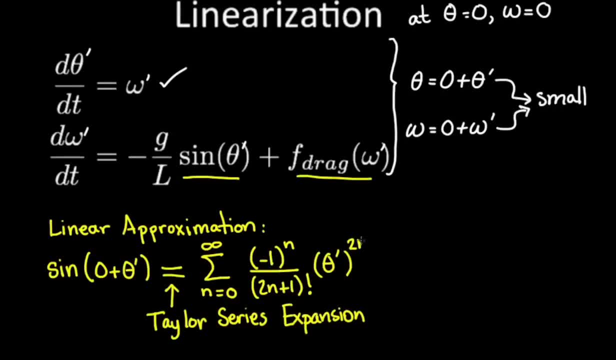 If we assume that theta prime is small, we can approximate sine of theta prime by theta prime: the deviation of theta from 0, by ignoring the higher order terms in the Taylor series, expansions of sine theta prime about 0.. Okay, Now what is the linear approximation of sine theta prime by theta prime? 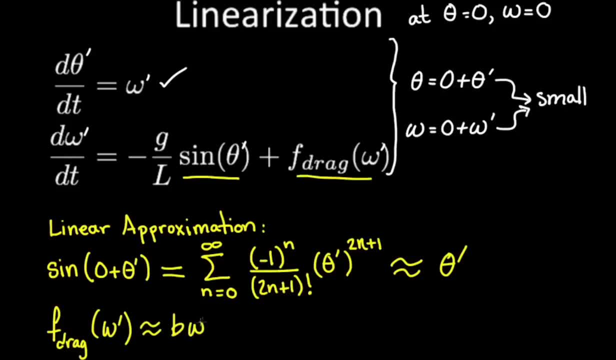 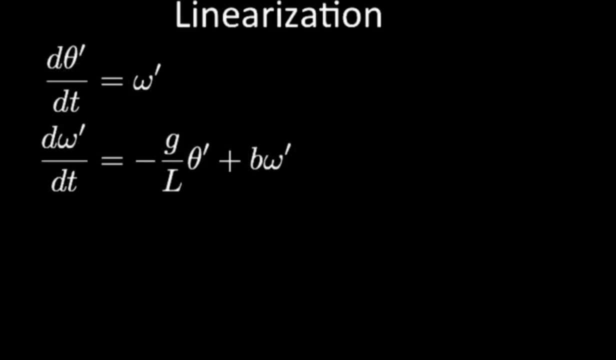 The linear approximation of sine theta prime by theta prime is 0.. Because we are linearizing near omega prime, sufficiently close to 0, the dissipation term is asymptotic to be omega prime, as mentioned previously. We then substitute these expressions into our dynamical equations to obtain: 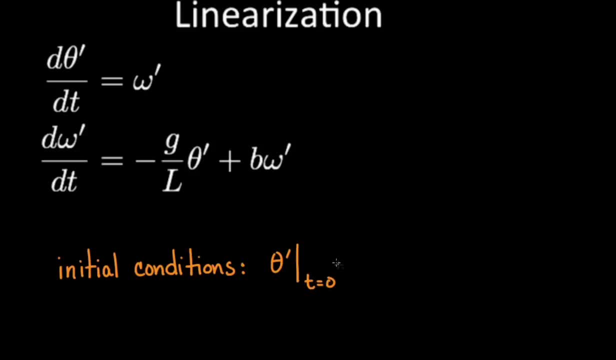 the linear equations indicated. We must supply initial conditions and the initial angle and angular velocity must be small in order for this linearized system of equations to be applicable. We now write the linear equations in matrix 4.. We now write the linear equations in matrix 4 in order to prepare for the next step. 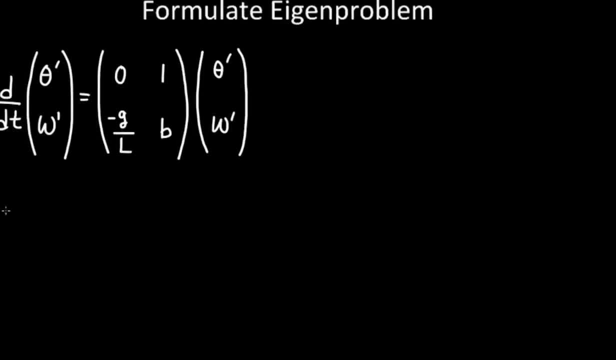 formulation as an eigenproblem. To do this, we assume temporal behavior of the form e to the lambda t. This yields an eigenvalue problem for lambda. Note that our matrix is 2 by 2, and hence there will be two eigenvalues and. 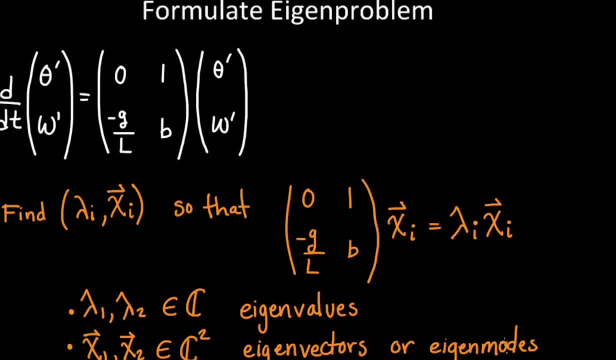 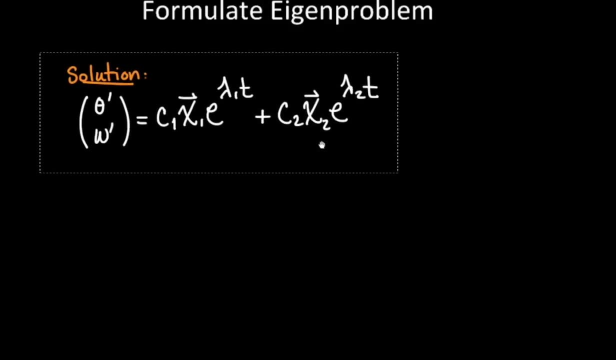 two associated eigenvectors or eigenmodes. Once we obtain the eigenvalues and eigenvectors, we may reconstruct the solution to the linearized equations as shown here. The constant c1, and c2 are determined by the initial conditions. However, to determine stability, a simple inspection of the eigenvalues suffices. 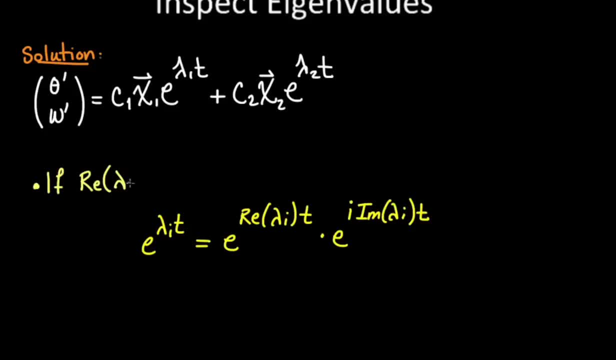 What happens to e to the lambda t when each of the eigenvalues has negative real part? Pause the video here We observe that e to the lambda t decays in this case and the system is stable. What happens if any of the eigenvalues has positive real part? 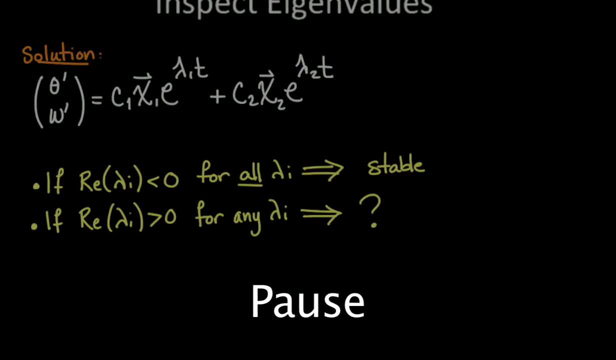 Pause the video. If an eigenvalue has positive real part, in which case e to the lambda t corresponds to exponential growth away from the equilibrium, the system is unstable. Note that even one eigenvalue with a positive real part is sufficient to deem the system unstable, since, sooner or later, 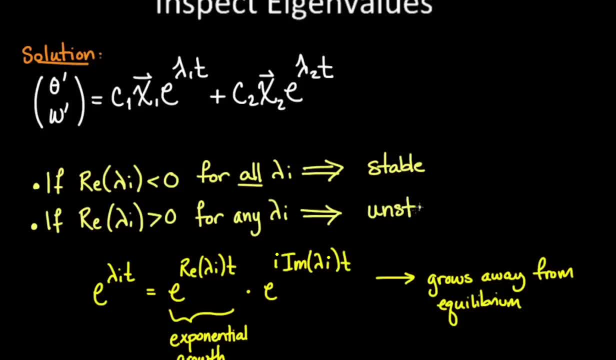 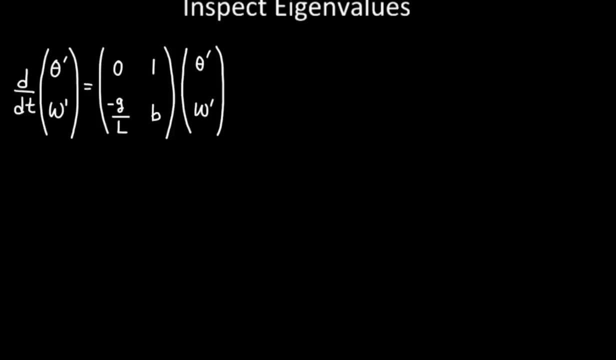 no matter how small initially, the growing exponential term will dominate. Lastly, if the real part of the eigenvalue with largest real part is 0,, in which case e to the lambda t is of constant magnitude, the system is marginally stable and requires further analysis. 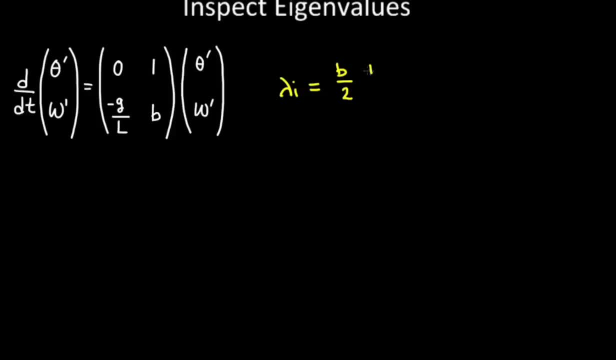 We now proceed for our particular system. For this problem, it is easy to find the eigenvalues analytically. We observe that both lambda 1 and lambda 2 have a small negative real part due to our negative damping coefficient b. Thus the system is stable. 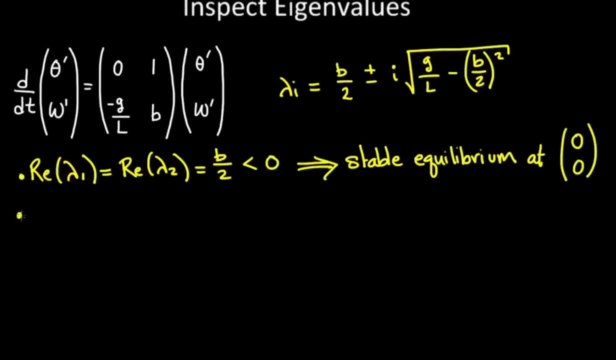 As we predicted, based on the physical pendulum For our experimental system, b, squared l over g, is much smaller than 1. And hence the damping does indeed have a small effect on the period of motion, If we recall the connection between the complex exponential and sine. 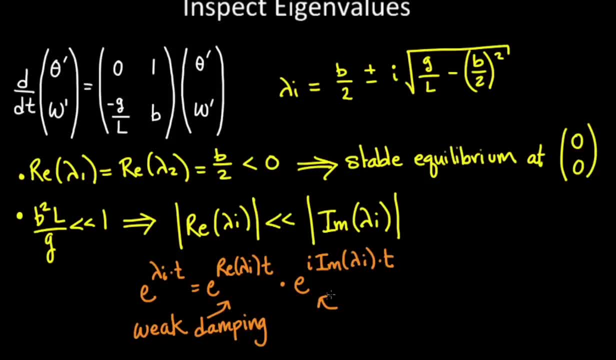 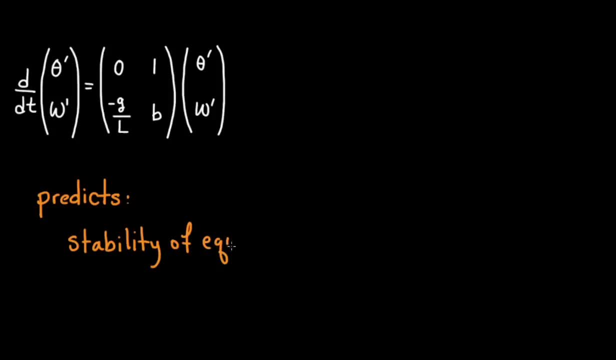 and cosine, we may conclude that the linearized system response is a very slowly decaying oscillation. This linear approximation to our governing equations- compare and subtract is a very linear approximation to our governing equations- can predict not just the stability of the system.